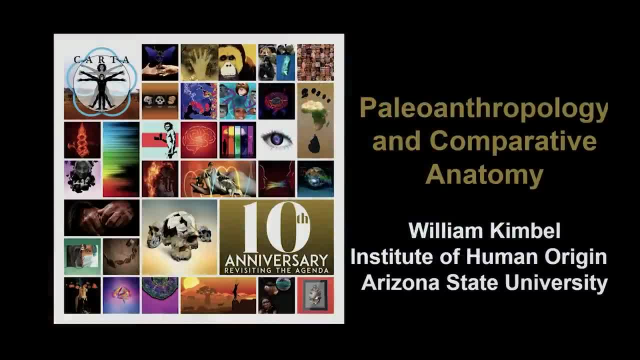 Good afternoon everyone. Sorry I can't be with you this weekend, But I'm pleased to be able to talk to you about paleoanalysis, anthropology, specifically what we know, what we think we know and what we've yet to fully. 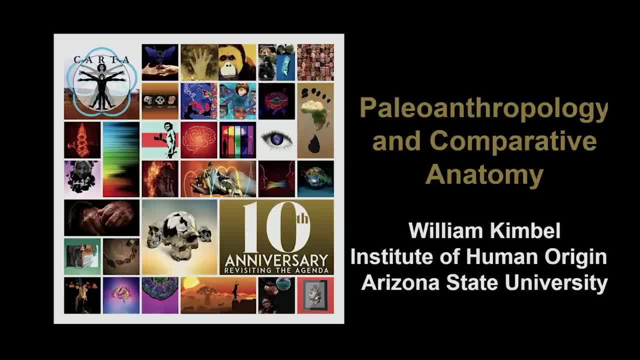 understand about human evolution from the point of view of the fossil record. Obviously, given the time constraint, I can't be comprehensive, but I'll try to be general rather than highly specific. I'll identify a few obstacles along the way and end with a short prescription for 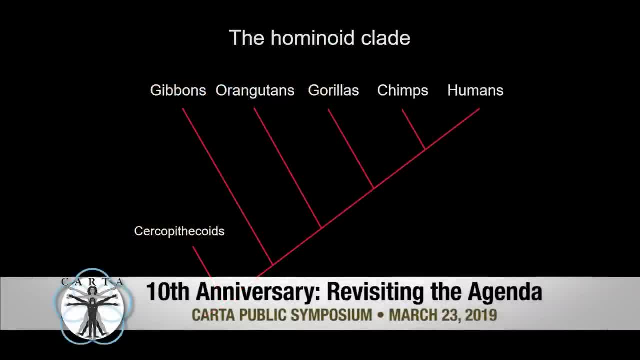 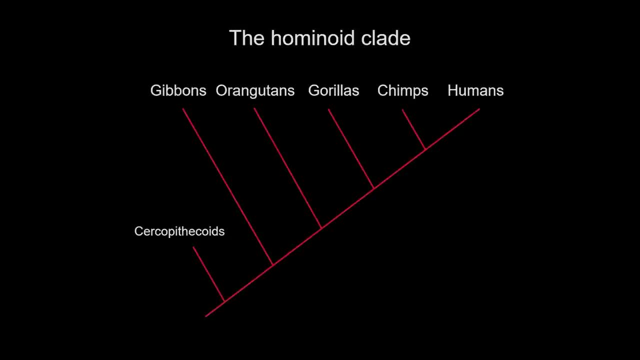 overcoming them. Perhaps the one thing we're most sure of about human origins doesn't actually come from the fossil record, and that is that chimpanzees and humans are more closely related to one another than either is to gorillas and other primates. This insight, of course, 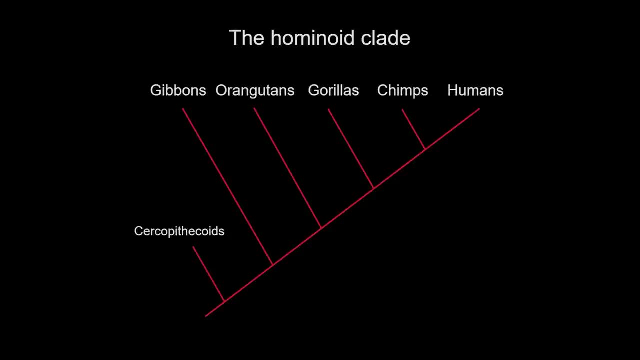 comes from the molecular evidence but is a central backdrop to any interpretation of the hominin fossil record. We're fairly sure that the human-chimp divergence occurred in the late Miocene, but that date has moved back some due to recent work on the slowdown of the molecular clock. 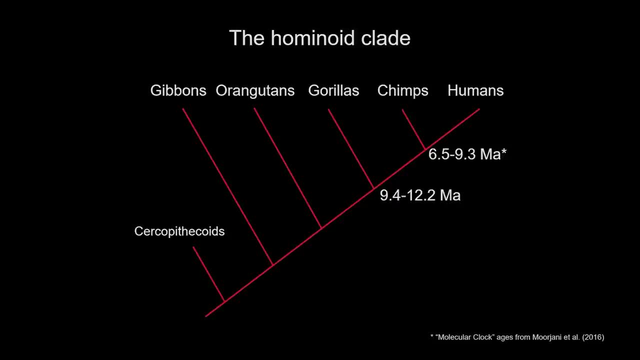 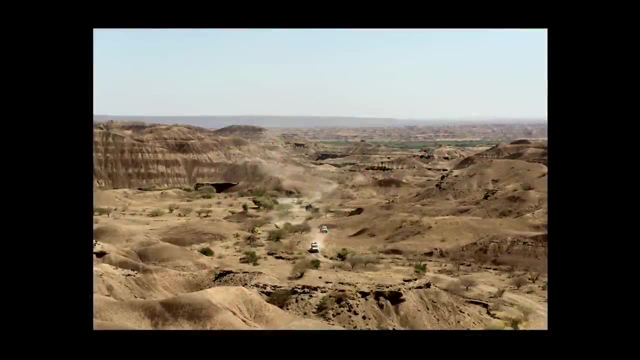 within hominoids and genome-wide analysis of variation and substitution. These dates are consistent with the known fossil record of early hominins, But nothing in the molecular record can give us the chronicle of events: what happened when, where and why. 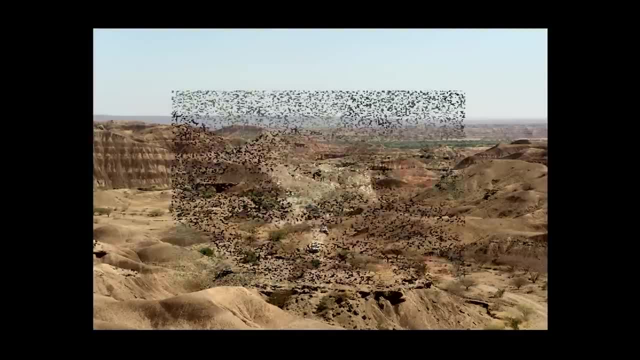 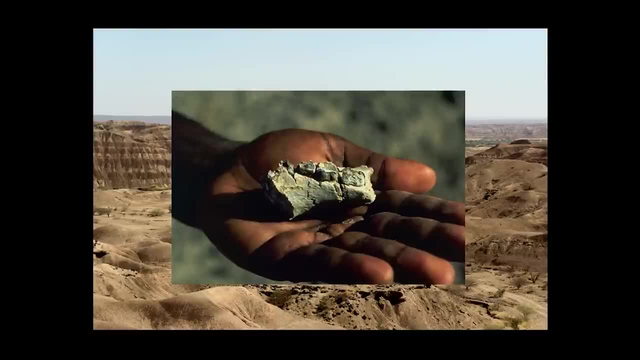 along the path from the last common ancestor to modern humans. For this we need strategically programmed fieldwork and a well-sampled, precisely calibrated fossil record. Here I've added to the statement of relationships two fossil tasks that are important to us. One is the question of how we can determine the 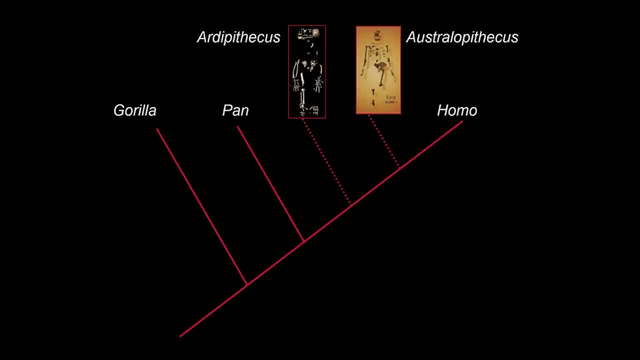 position of Ardipithecus, Ardipithecus and Australopithecus that contribute critical parts of the chronicle. Now I'm pretty confident in the basal position of Ardipithecus relative to Australopithecus and Homo, though I recognize some hesitation on this point by some in our field. 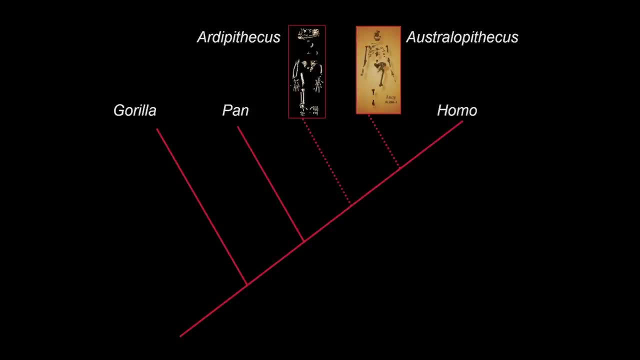 And the position of Australopithecus as a close relative of humans hasn't been seriously debated since the mid-1950s. Currently, Ardipithecus tells us that a trio of characters- part-time bipedality and part-time bipedality- are the most important, And that's because they're 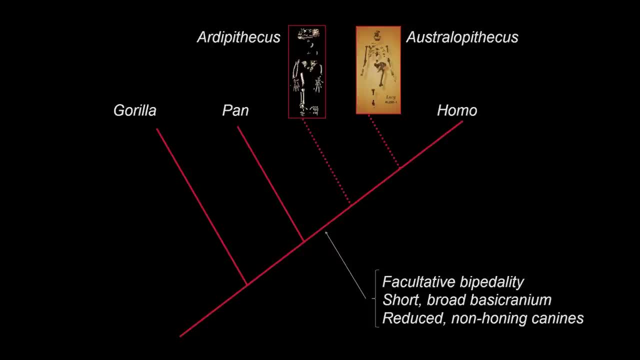 a broad, short cranial base with a centrally located foramen magnum and small, non-honing canine teeth are foundational specializations of the hominin clade. From the Ardipithecus perspective, Australopithecus appears to have undergone a radical makeover, with a number of 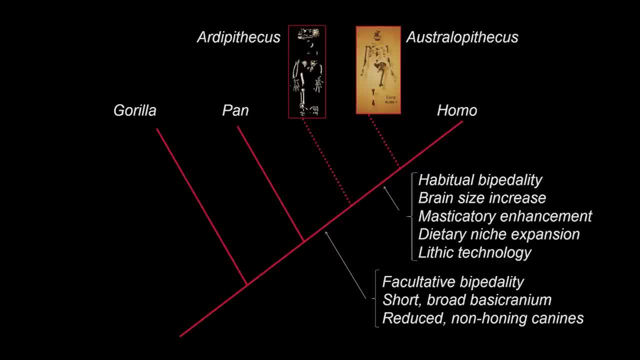 features such as lithic technology, a significantly enlarged brain and an expanded dietary niche that we've historically associated with the Homo lineage. In my judgment, though, the adaptive transition from Australopithecus to Homo is modest by comparison to that between Ardipithecus and Australopithecus. Now it's become fashionable. 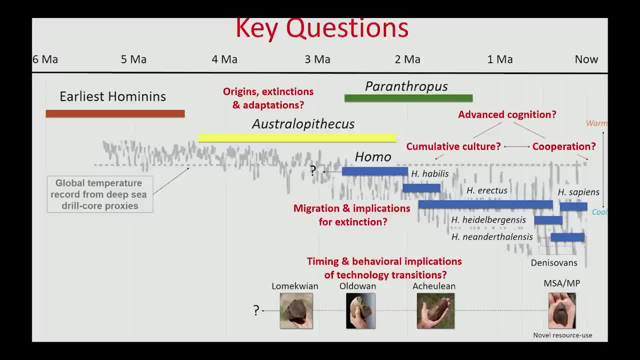 to attribute all of these changes and more speciations, extinctions, net changes in taxonomic diversity, the appearance of biological as well as technological innovations, to high-amplitude variation in global climatic cycles during the Pliocene and Pleistocene, within a strong trend. 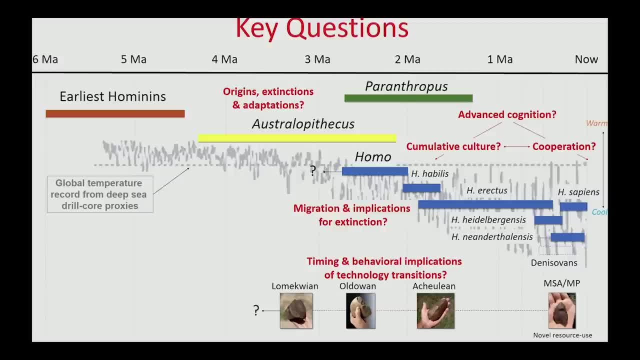 towards cooler, drier conditions, And I think that's a very important point. And I think that's a very important point. And I think that's a very important point. But early hominins weren't adapting to climate change. They responded to changes in local 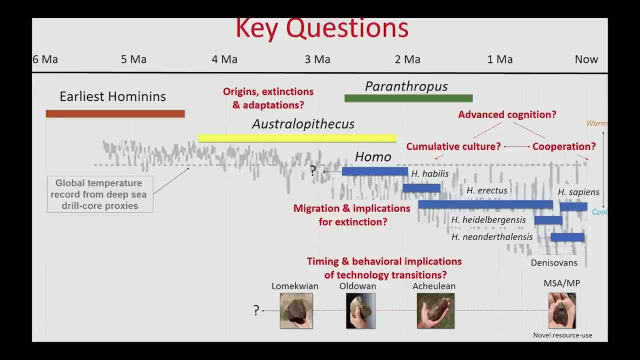 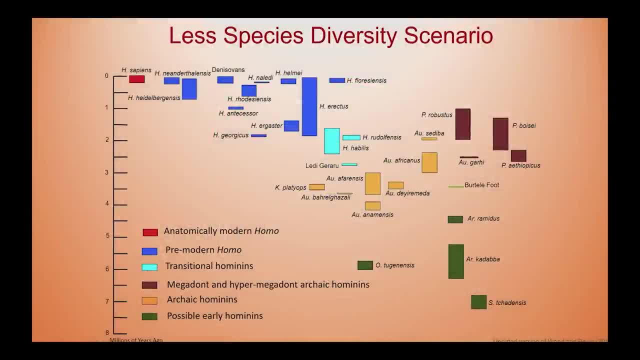 understanding of how large-scale climate changes can affect the environment. We do not have a full understanding of how large-scale climate changes can affect the environment. We do not have a full were rigorously applied to the hominin fossil record, perhaps 20 to 25 percent of the currently. 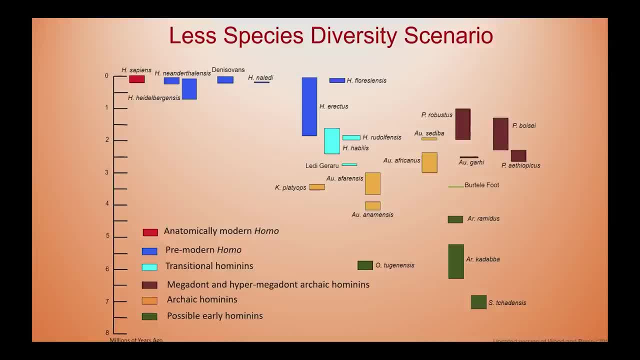 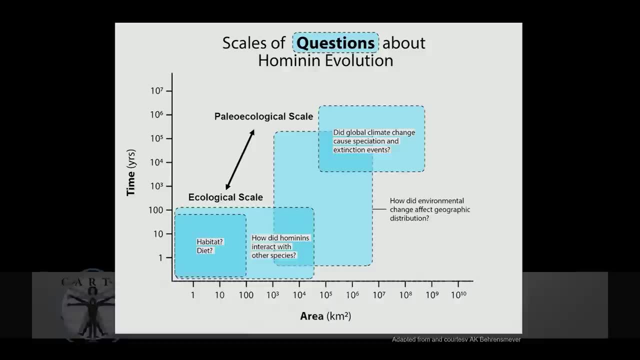 named species would lose their identities as independent twigs on the tree of life, and some of my colleagues would argue that I'm still not being conservative enough. Now I want to say a few words about another major obstacle, one that does not have to do with our 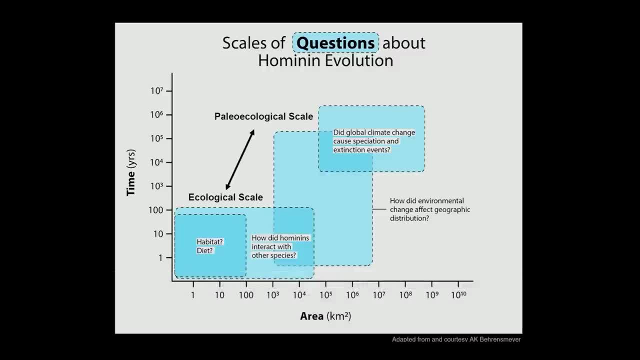 handling of the evidence per se, but instead concerns the disjunction between the scale of the questions we ask and the scale of the evidence we use to attempt to answer them, And here I want to acknowledge Kay Behrensmeyer of the National Museum of Natural History. 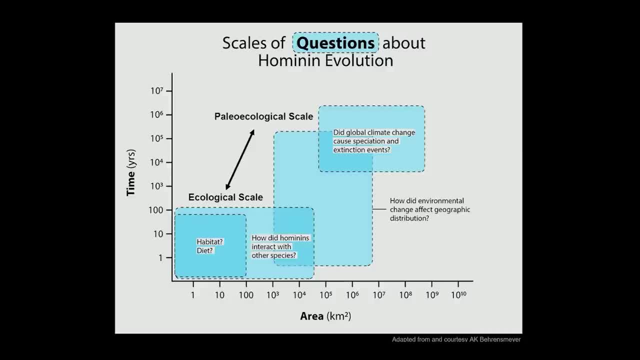 whose important work on this subject deserves much better treatment than what I can offer in the next few minutes. Here are plotted the spatial temporal realms of some of the major questions we ask about the hominin fossil record, ranging from the truly global scale on the order of hundreds of thousands to millions of years of time to similar large. 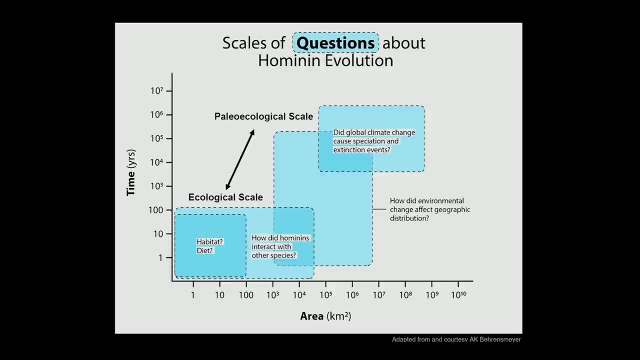 space-time scales and to the scale of the evidence we use to attempt to answer them, Down to what we might call local or ecological scale questions concerning population responses to environmental change. Many of the phenomena of human evolution we wish to explain are located on the ecological scale: speciation, population dispersals. 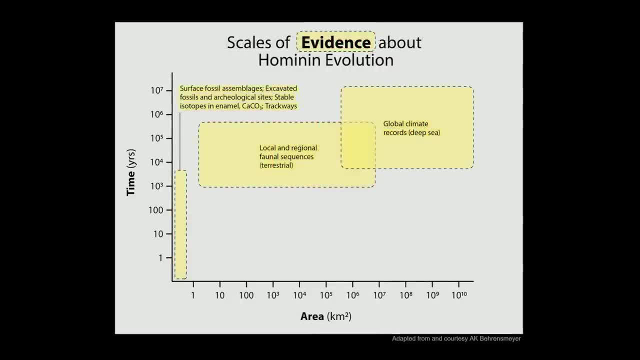 origins of adaptations, etc. Accordingly, it would be extremely helpful if at least some of the evidence from the fossil record aligned with those questions. Unfortunately, for the bulk of the record, that is not the case On the ecological scale in which many of our most. 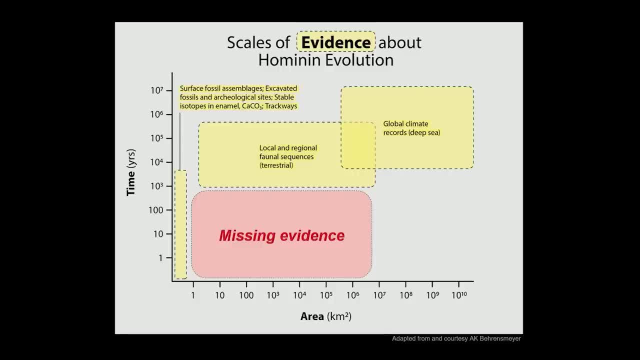 interesting questions reside. we're usually short-changed when it comes to the data. We are squeezed between, on the one hand, the spatially narrow window afforded by individual localities monitored over relatively short time spans- snapshots, really- and, on the other hand, 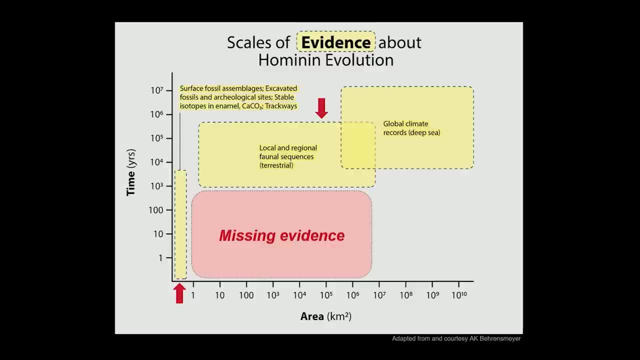 faunal assemblages that are almost always temporally mixed across landscapes, aggregating individuals from different places. On the other hand, we are squeezed between, on the one hand, different biological populations and ecological conditions. Well, this sure sounds like a gloomy prospect for paleoanthropology. 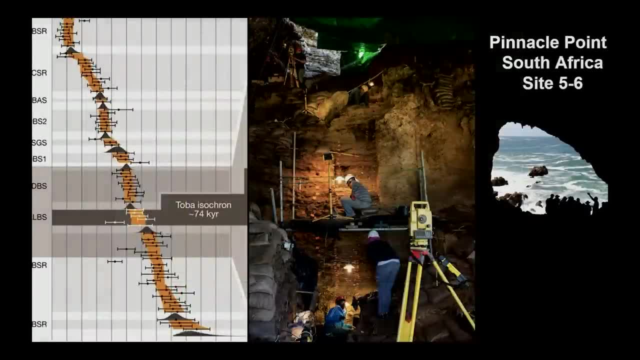 But there are exceptional cases, like my colleague Curtis Marion's excavations in South Africa, where one of his cave sites preserves a continuous, exquisitely detailed, virtually landscape-scale paleoclimatic and archaeological record of Middle Stone Age humans. 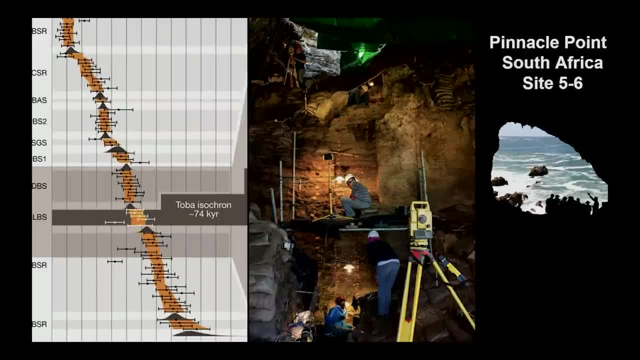 in a coastal marine setting between around 90,000 and 50,000 years ago. The sequence includes traces of the mammoth Toba volcanic eruption and presents a rare opportunity to study how early humans responded to an environmental crisis in ecological time. 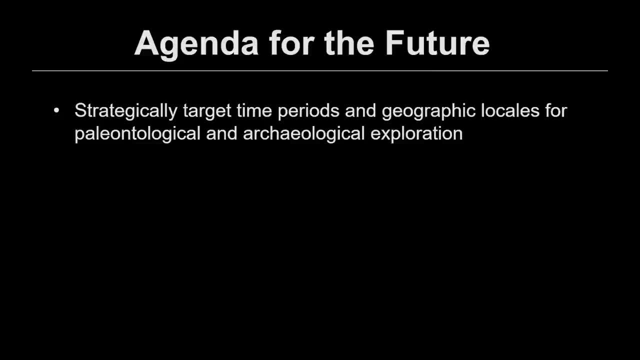 But this is, as I say, an unusual circumstance. So where should we go from? here? I offer a short list of agenda items that by no means exhausts the list of important tasks for the next generation of paleoanthropologists. It's trite to say, but we need more evidence. 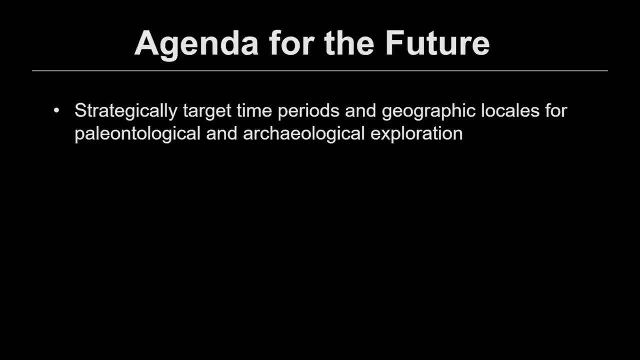 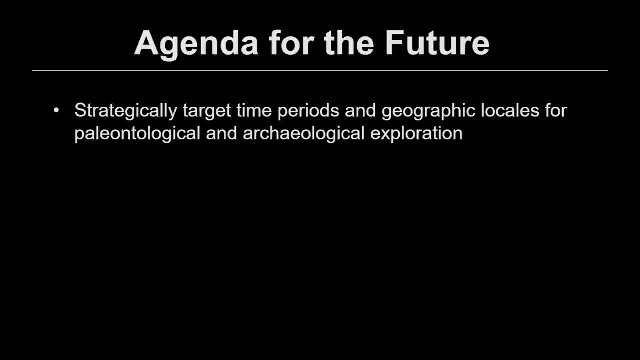 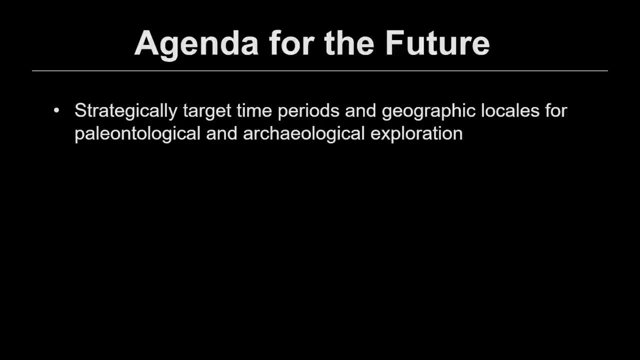 from fresh paleontological and archaeological discoveries. I have my own favorite gap in the African fossil record between 3 and 2 million years ago, but there are others equally worthy of time and resources, like the entire Pleistocene of Central Asia, for example. 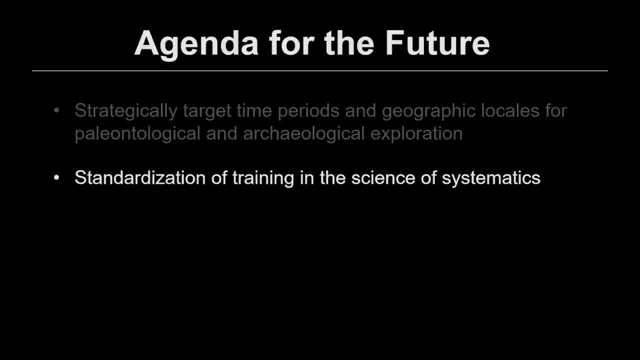 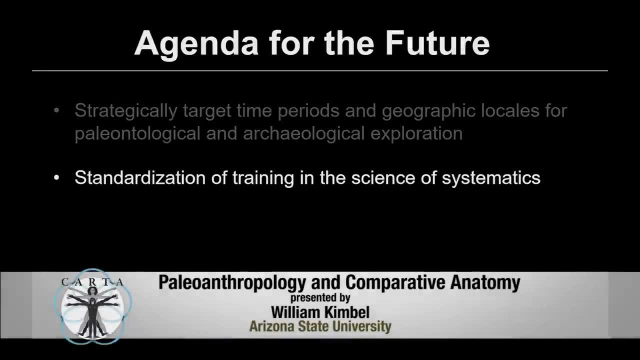 I'm going to sound awfully old-fashioned here, But students in human origin science need more rigorous training in the basic principles of zoological systematics. Systematics is the bridge between the field and the laboratory, and I think paleoanthropology as